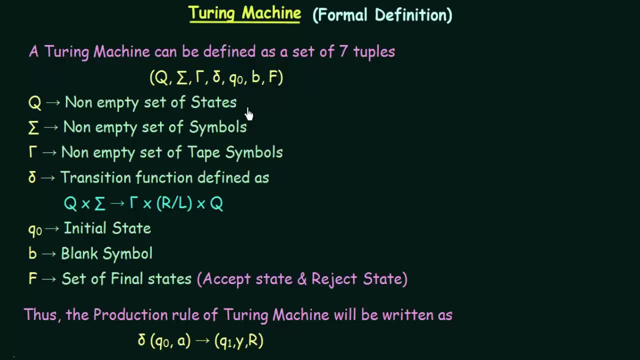 Even in finite state machines and push-turn automata also, Q was a tuple that is used to represent the non-empty set of states, So that is the same even in case of Turing machines. And then we have Sigma, And Sigma also just like the other machines that we have. 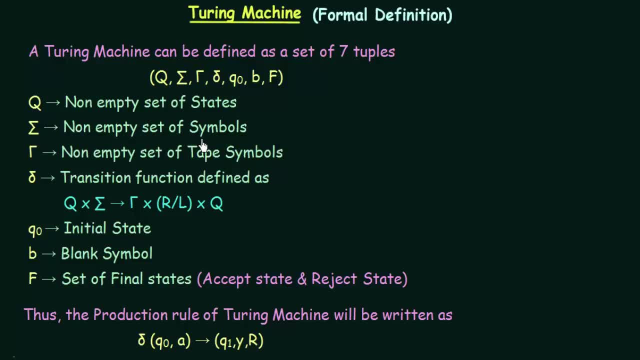 it represents the non-empty set of symbols, Or we can say it is the symbol, It is the set of input symbols that we have in our Turing machine, And then we have Tau. Now, Tau is something different from finite state machines and push-turn automata. 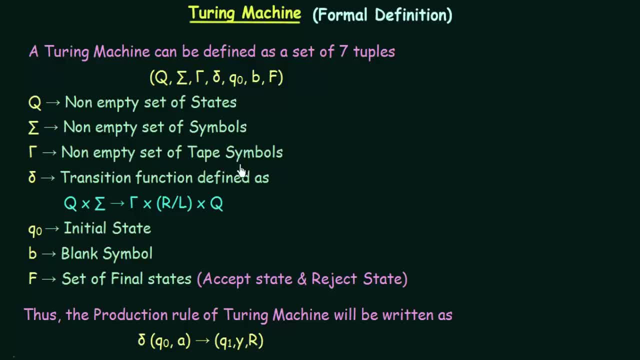 And what is it? It is a non-empty set of tape symbols. So when we studied the introduction of Turing machines, we saw that Turing machine has something known as the tape. What is a tape? It is an infinite sequence of symbols. 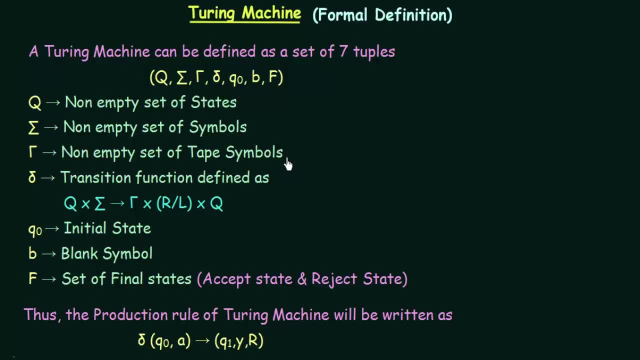 So those symbols, that means the tape symbols. they are represented by this tuple Tau, So it is a non-empty set of tape symbols. And then we have Del, which is a transition function, And we know that transition functions are there even in finite state machines and push-turn automata. 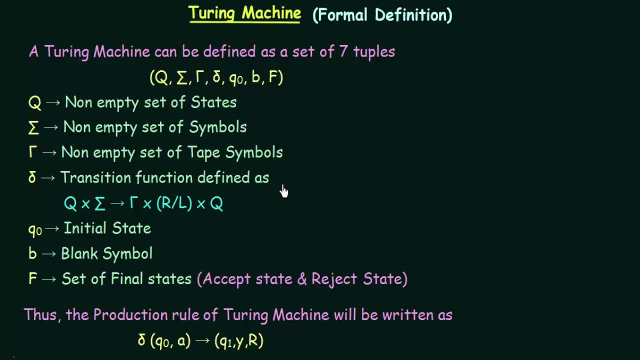 And they are defined in different ways according to how the machines work. So, in case of Turing machine, we have the transition function, Del, which is defined like this: Q cross Sigma to Tau cross R or L L cross Q. Now let us see what this actually means. 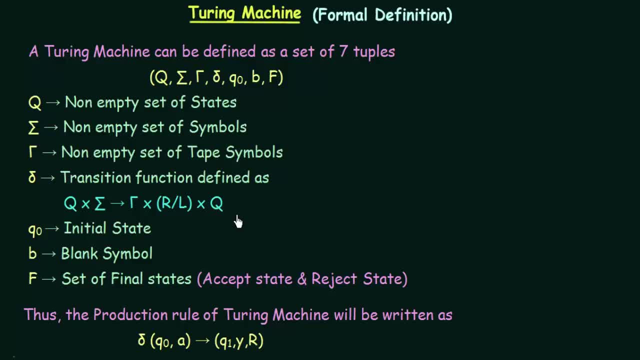 So we know that in Turing machine we have states and then we have our input symbols And we also have the tape symbols. And here this means that when we are on a particular state, on getting a particular input symbol, we write something into the tape sequence. 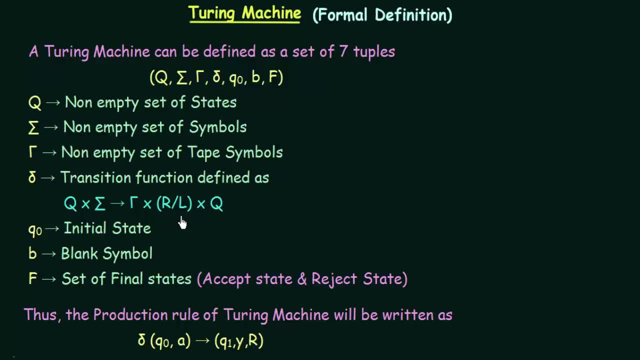 and we move either right or left on the tape And then we go to the next state. So that is what we mean by the transition function Del in Turing machine, Because that is how the Turing machine actually takes transition from one state to another. 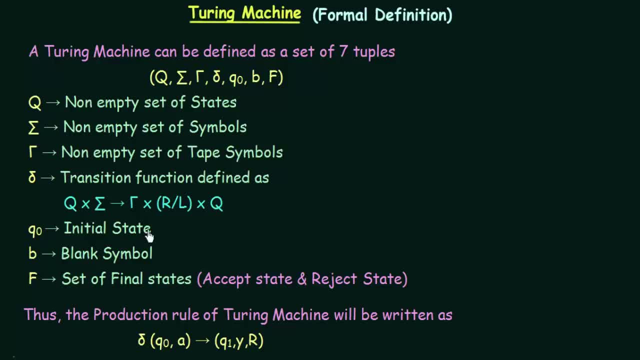 So this will become more clear when we take our examples. And then we have Q0, which is the initial state. So Q0 is the initial state or the starting state. And then we have B, which is the blank symbol. So if you have seen the introduction of Turing machines, which I have already discussed, 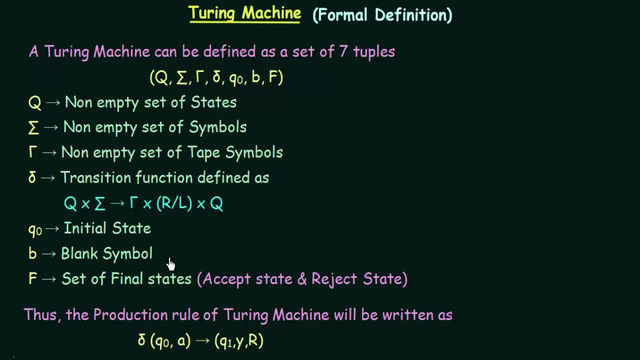 we saw that in the tape we have a special kind of symbol known as the blank symbol. And what is the blank symbol? It is a symbol that is used for filling up the empty spaces in our tape sequence. And then we also said that this blank symbol does not belong to the set of input symbols that we have. 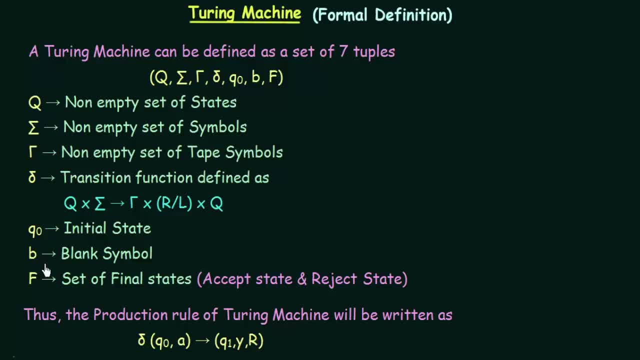 That is why I said blank is a special symbol And that is why we have a different tuple that is used to denote the blank symbol, which is B, And then we have F, which is the set of final states. So even in the introduction I already discussed that- 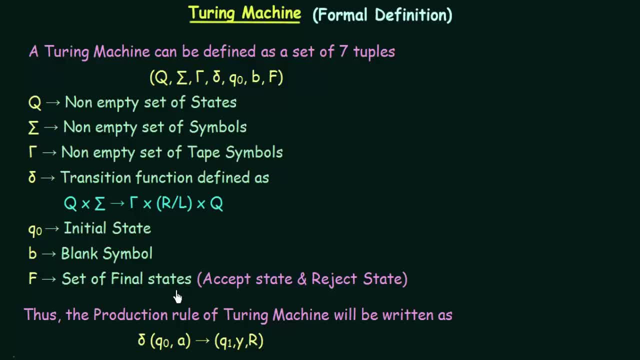 in Turing machine there are basically two kinds of final states. One is the accept state and another one is the reject state. So F represents the set of final state. So these are the seven tuples that are used to define a Turing machine. 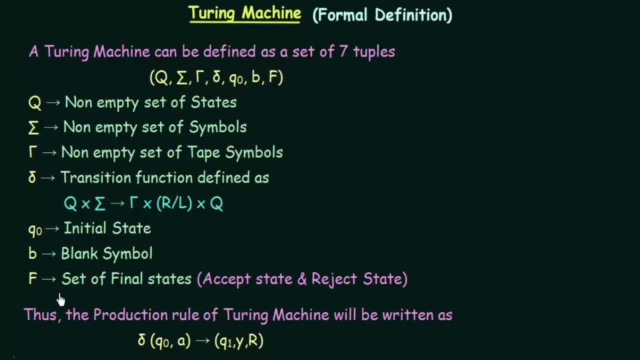 Now let us see how we can write the production rule of Turing machines. So the production rule of Turing machines. It can be written like this: And what does this mean? This means that initially we are in the starting state Q0.. 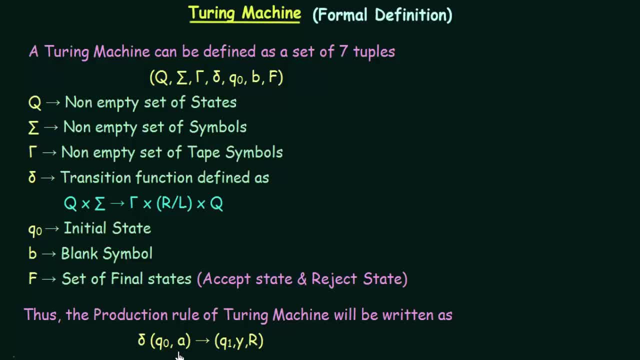 And on getting a particular input symbol, it could be anything, So we just represent it by A over here. And on getting this particular input symbol, it goes to another state, Q1. And it writes the symbol Y onto our tape, And then we move either right or left on our tape. 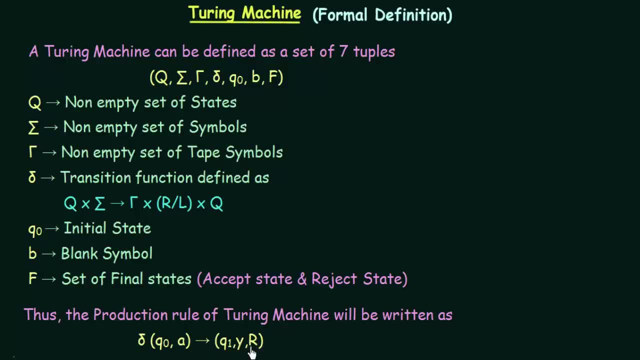 So here it is. Here it says it is moving right. So this is just an example and it shows basically how the production rules of Turing machines are written. So even when I explain the transition functions, it should be clear to you how the transitions are taken. 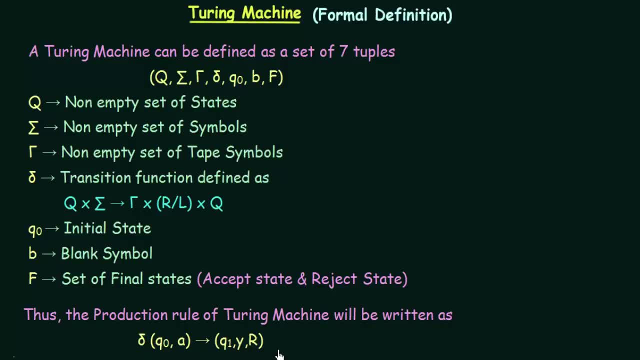 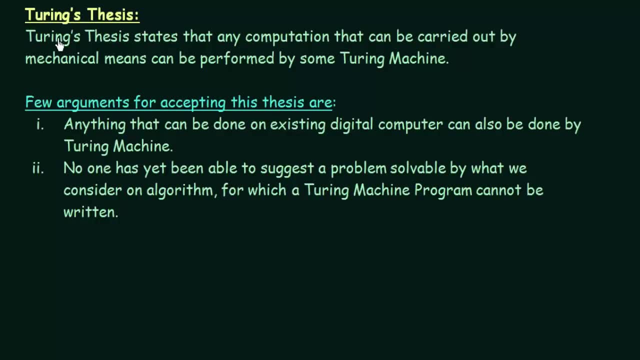 And if you understand this, this production rule will be clear to you. Now the next thing that we need to discuss about is Turing's thesis. So let us see what this Turing thesis says. Turing thesis states that any computation that can be carried out by mechanical means can be performed by some Turing machine. 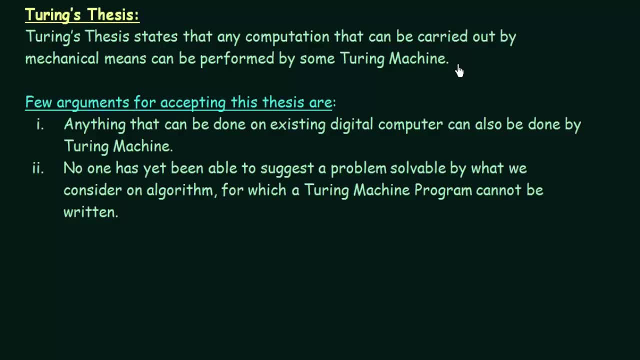 So Turing thesis says that if there is any computation that can be mechanically performed, then that computation can also be performed by some Turing machine. So from this you can understand how powerful a Turing machine actually is. So we have discussed about other machines in this course of lecture series. 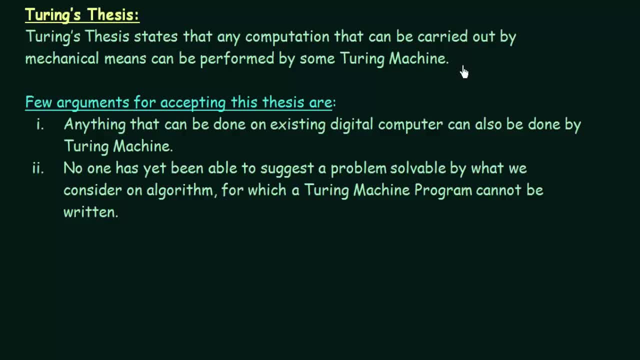 Like finite state machines and push-on automata And we saw that, how limited they are and what are the limitations that they had. But seeing this Turing thesis, you can understand how much more powerful a Turing machine is as compared to finite state machines and push-on automata. 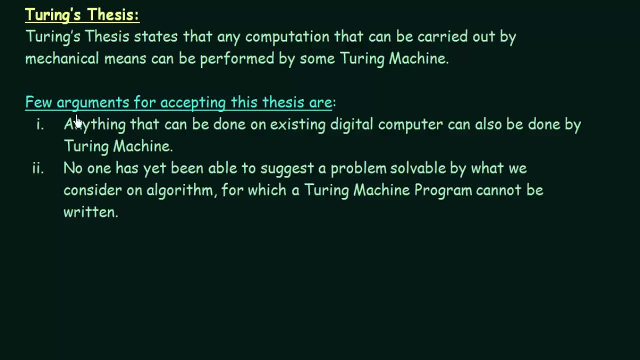 Now this is the Turing thesis that we have, and there are few arguments for accepting this thesis. Now let us see what are the arguments that are used to accept or support this Turing thesis. Number one: Anything that can be done on existing digital computer can also be done by a Turing machine. 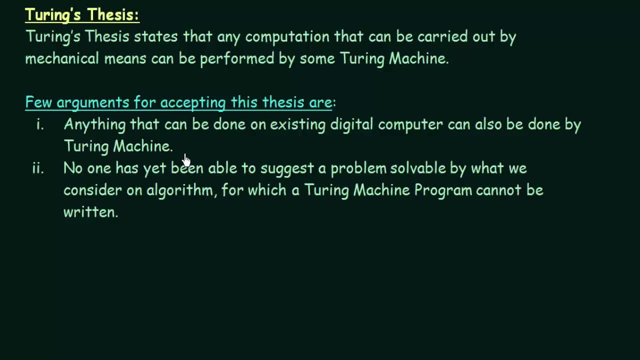 So any computation that we can do on an existing digital computer that we have today, that can also be done by a Turing machine. So we see how powerful Turing machine is. And then number two: No one has yet been able to suggest a problem. 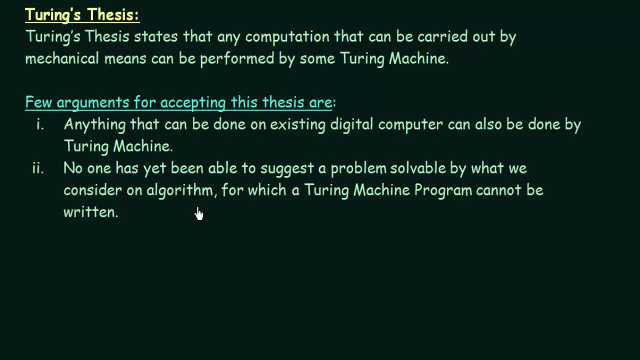 solvable by what we consider an algorithm, for which a Turing machine program cannot be written. So this means that if there is a problem that you have and if you are able to write an algorithm for solving that problem, then you will also be able to design a Turing machine program. 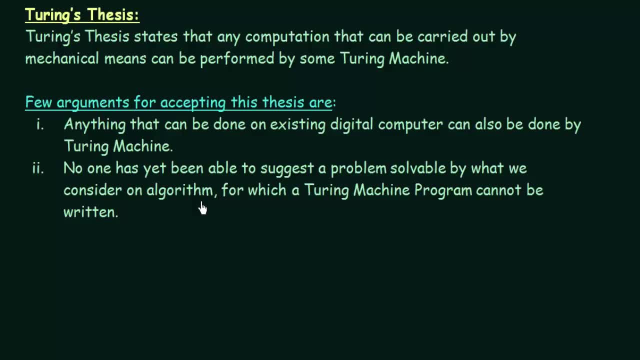 which can be used to solve a same problem. So till now nobody has been able to suggest any such kind of problem whose algorithm can be written but cannot be solved by a Turing machine. That means if you are having the algorithm, if you are able to design the algorithm for a problem. 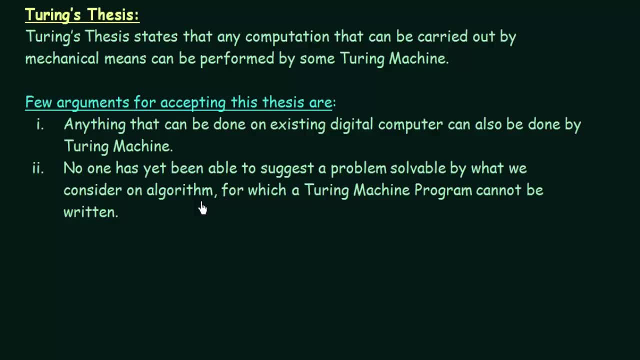 or for solving a problem, then that can also be solved by a Turing machine. So that again shows how powerful a Turing machine is. And these two arguments: they support our Turing thesis, which says that any computation that can be carried out by mechanical means.